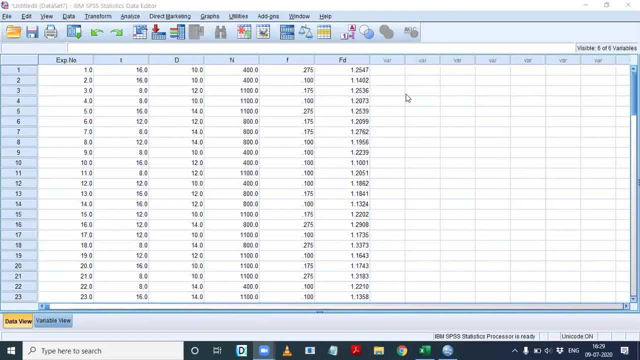 a univariate and a multivariate is that in a univariate there is only one variable and in multivariate there are more than one variables. in the data that we have Now, this particular data set that I am using is called a multivariate regression model. So this particular data set- 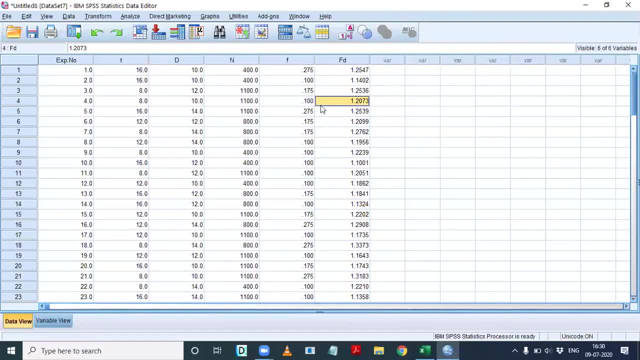 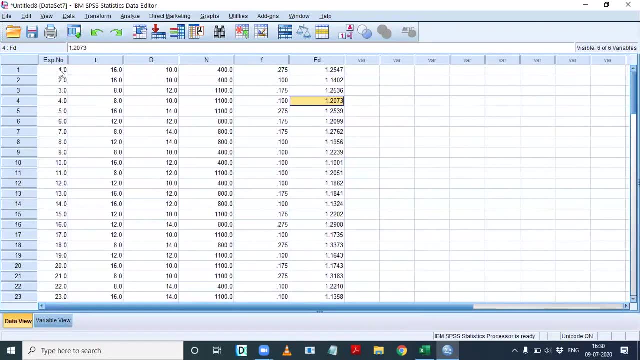 that I am using belongs to a machining operation that I have conducted for one of my research papers, And what exactly is happening here is that I have around 81 different experiments that I have conducted. There are 81 different experiments which I have conducted and these 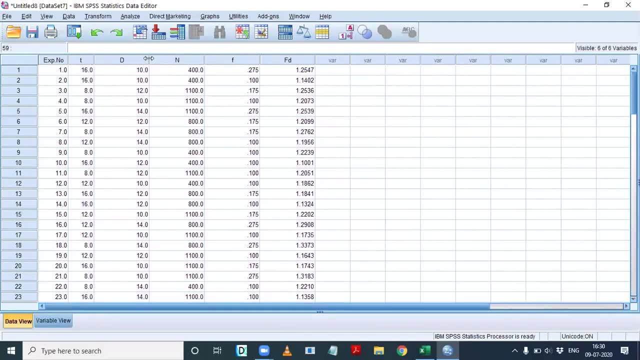 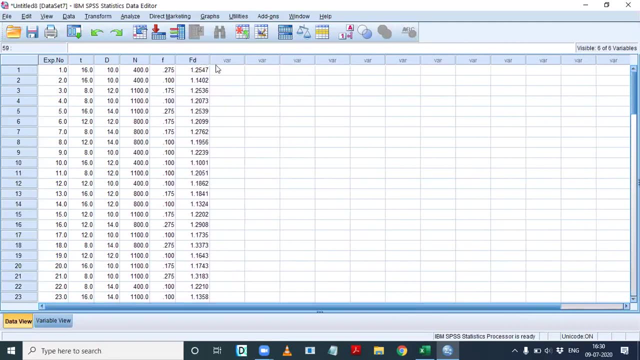 81 different experiments can now be classified into this different number of variables. This is the output. So T, D, N, F, these are the variables. Let's not go into the details of what these variables are. Just understand that these are the variables, and this is my. 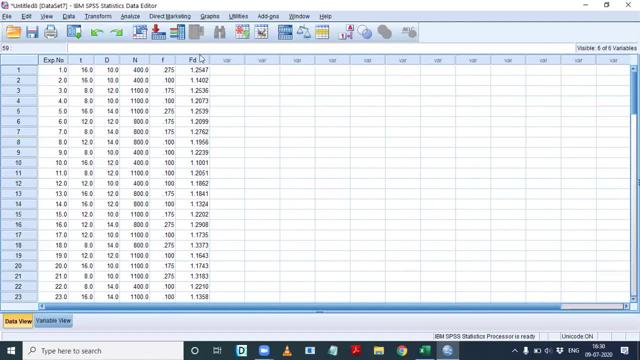 output. This is my objective, or this is the response that I want to predict. FD is the response that I want to predict, and T, D, N, F are the variables that affect the FD. So, basically, what we are trying to do here is that we are trying to build a regression. 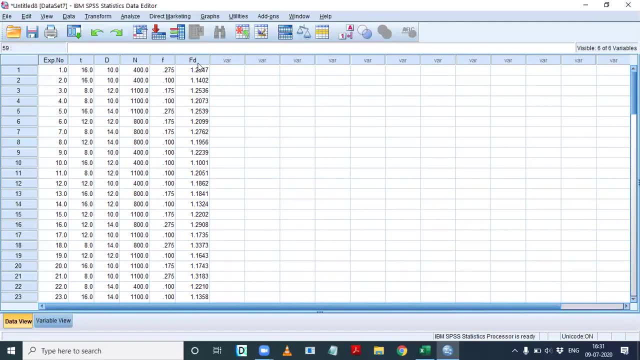 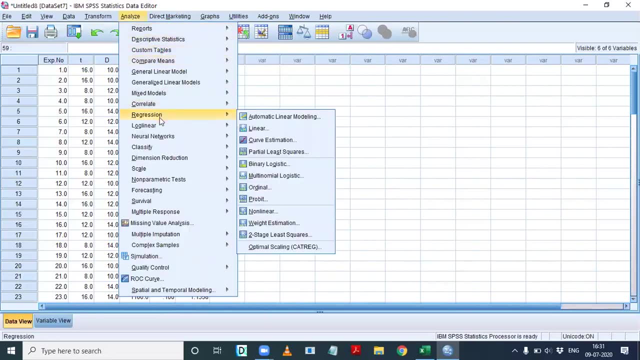 model where FD is a function of T, D, N, F. So now, how to do that? We will go to analyze, We will go to regression. So, as you can see, there are a number of different regressions here. So right now I am concerned only about linear regression. So let me go and let me. 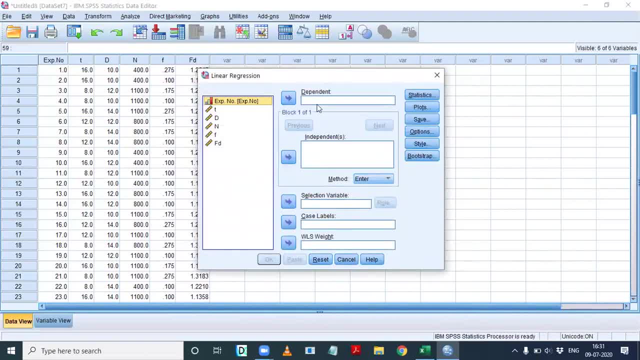 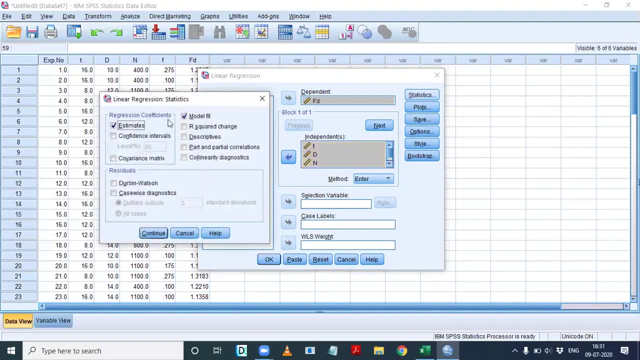 go to the linear regression. So in the linear regression I am going to go and select my response, which is the dependent variable, And all these things are my independent variable, which will go on here. So now I can go to the statistics and now I can decide what I 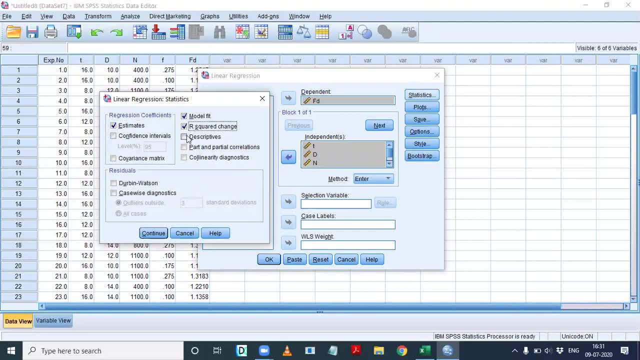 want to see. I want to see the R square changes. I will explain you what R square changes is. If you want to see the descriptors, you can see. these descriptors are nothing but the mean median quartile. All these kind of information will be displayed if you switch. 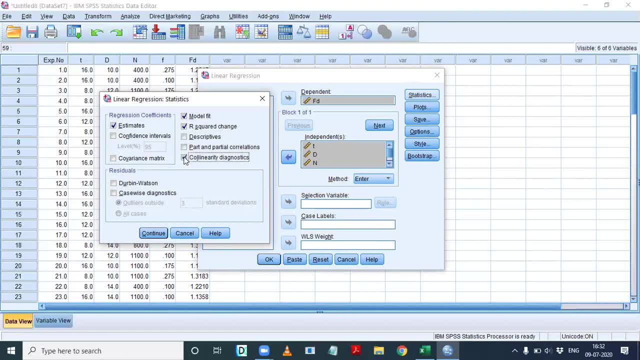 on the descriptors Again, if you want to do a collinearity diagnostic- there is a number of different variables- We will go to theiling And this way this will go on here. So now that also you can do. and if you want to do part and partial correlations, that also you can do. 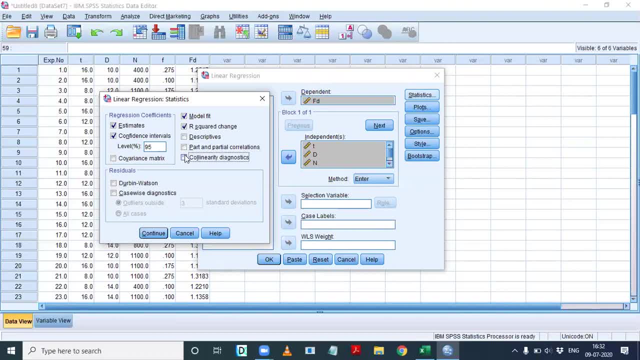 and i suggest you should let's switch both of them off for right now. uh, we do not want to. okay, we did not explain everything right now, so it'll go on step by step. so we want to. you want to specifically look at the confidence intervals of 95 if you want some other percentage, suppose. 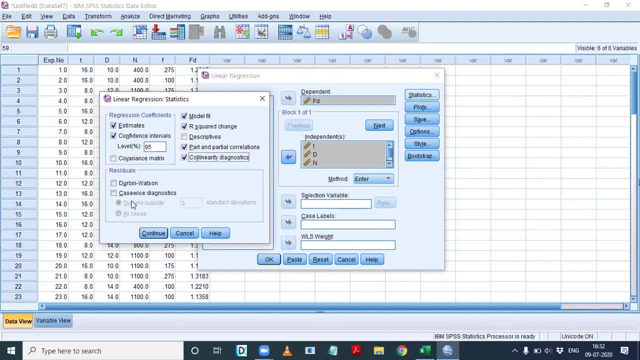 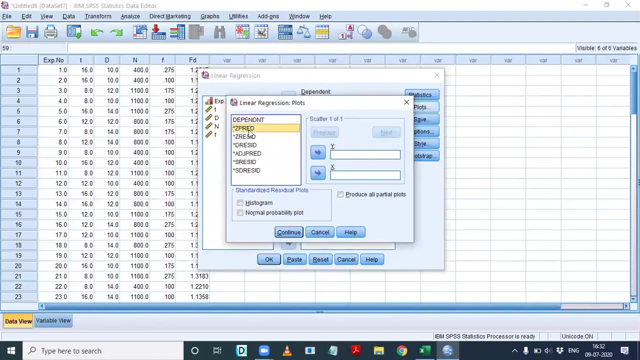 a 99 percentage. you can go and click on me if you want to do some analysis on the residuals, like the durban durbin watson test. you can go and do that, and uh, this is about it. and then here i probably told you that you should look at the jet predicted versus the jet residual. okay, 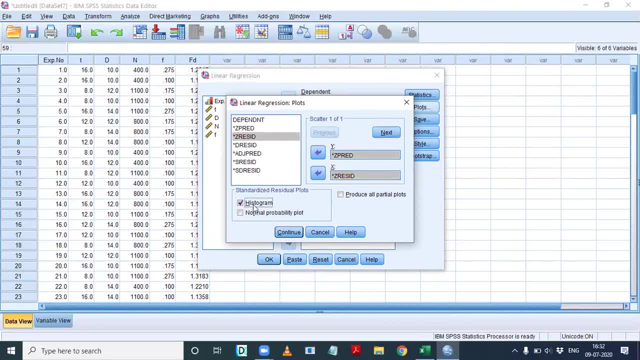 this is nothing but the predicted versus the residual and i want to look at the histogram of the residuals and i want to look at the normal quality part of the residuals. okay, i'll tell you why. i want to look at all of them, okay, and then i can go and in the options. 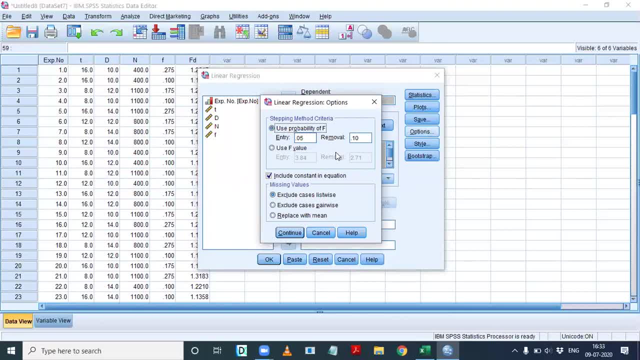 i have the stepping method criteria here. so basically, what happens here is that if you have any entry, if you have any term or any variable that has p value of less than 0.5, it will be entered, and if it has a p value of more than 0.1, then it will be removed from the model. okay, so we, we are using this particular 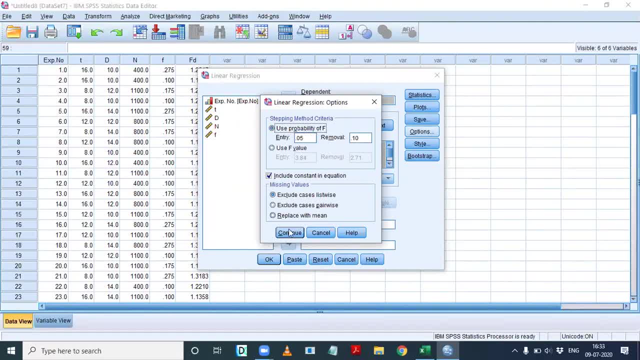 formula, that is the use probability of f. we are using this one and if you want, you can go and use something else also. okay, here again we want to look at, uh, if you want to, what do you want to save? okay, so, basically what, what do you want to save here? so you want to probably look at the 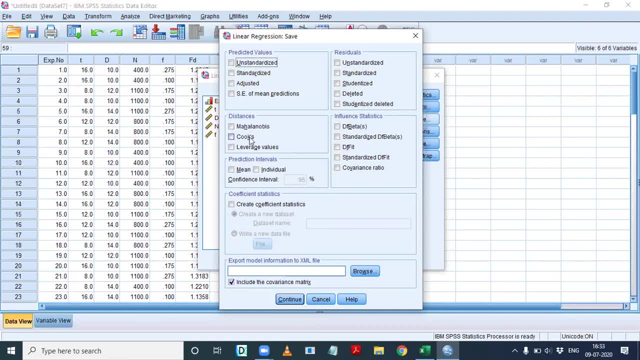 cook's distance or the monogamous distance and all that. so these are done to find out some uh sort of uh the data, how they are normal or not. so we look at all these distance and my anomalous distance and leverage value distance and all that uh so right. 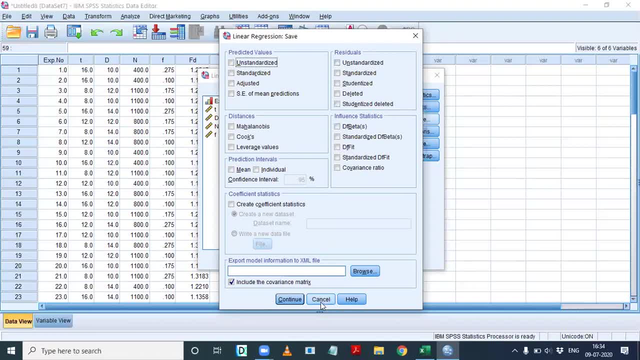 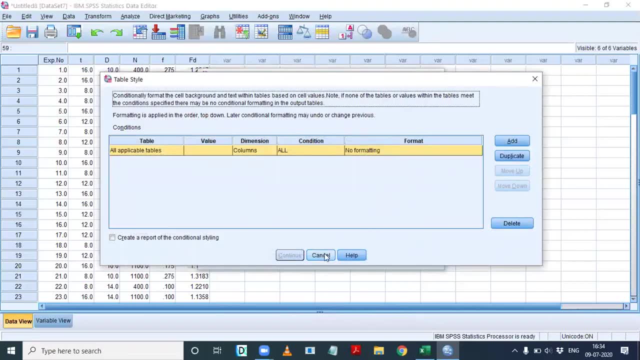 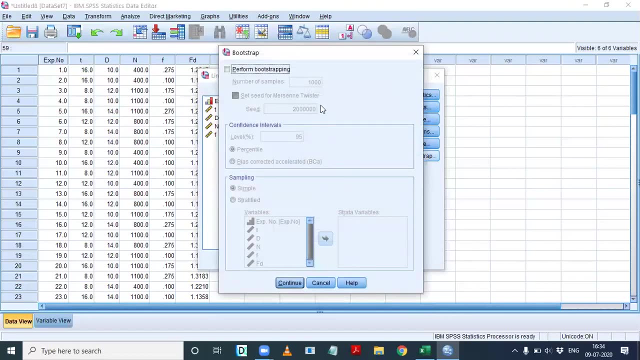 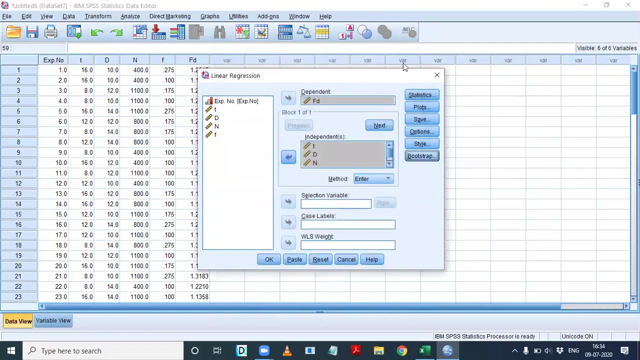 now, i'm not interested in having all of this. so let's uh cancel this and let us go to style and see if there is anything else to do here, okay, and in the bootstrap, uh, what is basically bootstrap, okay, uh, okay, we can just cancel this for now and then, uh, we can go on and we can click, okay. 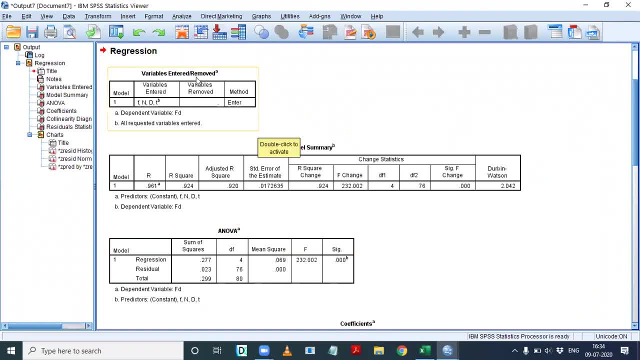 okay. so, as you can see here from here the regression begins. so so, as you can see from the uh tree that you see in the left side, quite a amount of, quite a lot of data or quite a lot of analysis have been done on the uh data that we have seen so far. so i'm going to go ahead and 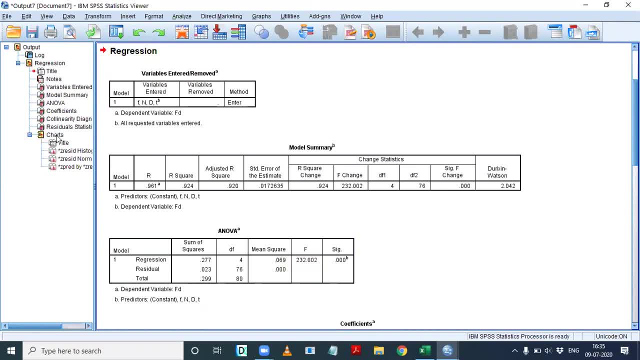 look at the data set that we have just injured it. okay, the on the data set. a lot of analysis have been done and these are some of the outputs that are displayed here. okay, so let us go and look at them one by one. for example, the first one that you see here is that the variables- 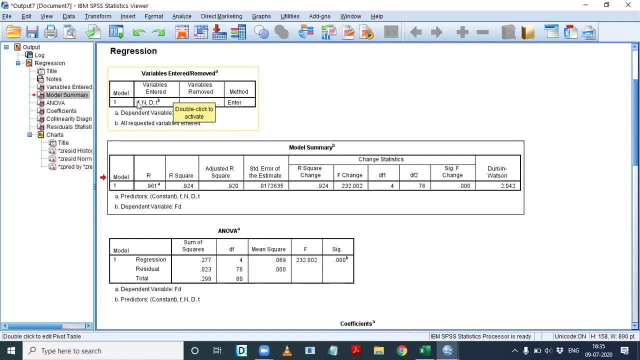 entered or removed. so we are using the enter method, which means we are forcing each of them to enter into the regression. okay, f and dt: these are the four variables and we are forcing each of them to be entered into the uh, into the regression model. okay, where fd is a function of f and dt, okay. so when f and dt are, 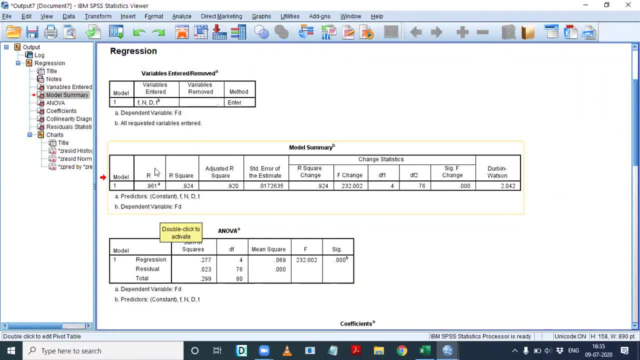 all four different individual parameters. now you have the uh correlation here, or the multiple correlation here, which is 9.61- okay, it's, it's a pretty high number. and you have the r square here, which is around 0.92 or 92 percent, and the adjusted r square is also around 92 percent. so 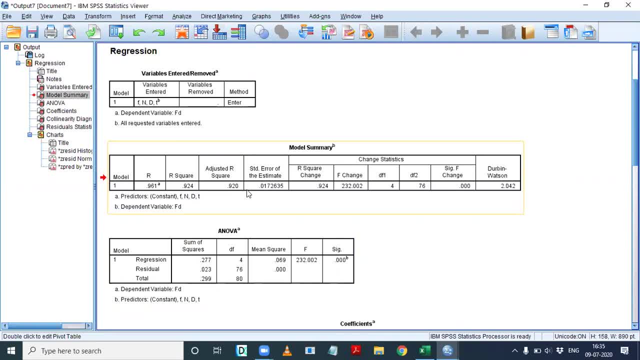 you can see that, uh, the model that you have built, or the regression that you are built, is able to explain 92 percent of the variance, 92 percent of the variance in the data that you have. okay, and you have the standard error of the estimate and you have the r square. 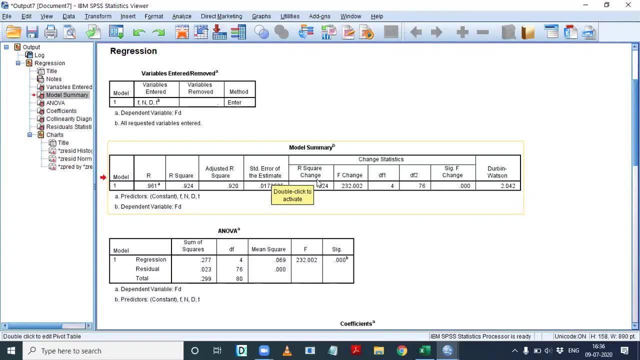 changes here. so what is r square change? r square changes nothing, but whenever you insert a new quantity. okay, for example, suppose initially you started with a regression model where you have only f in the regression model and next time you inserted an internet relation model, next time you inserted the. 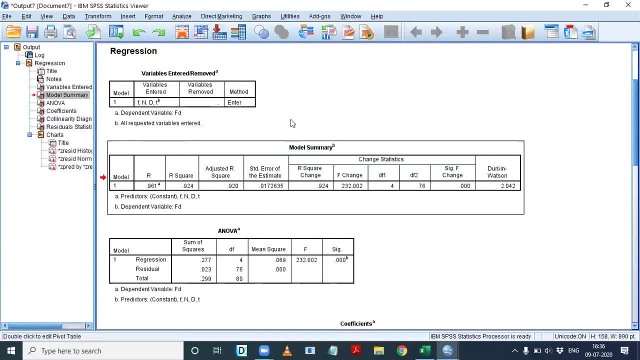 integrity. next time you inserted the integral regression model. when you do this step by step, what happens is that every time you add a variable or delete a variable from the regression model, there will be some changes in the uh in the regression- okay, and dead changes will be recorded here, okay. so it may be high also, it may be it may be towards downhill side. 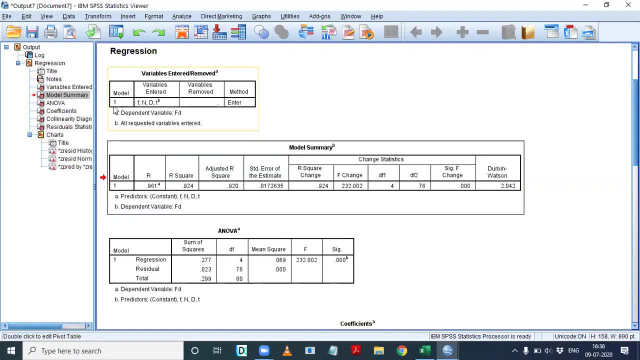 also. it will show it off inside also, but in this case, you can see only one. only one step was created is, which is why you can see one here. okay, only one step was there, and since all of these are the covariates or the predictors, all of them were entered once. 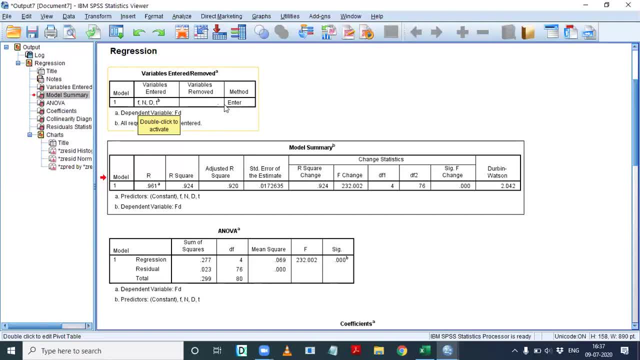 just in the single kind of statement all of them were entered and so so there is no R square change here, because there is no second step. if there were any second step, so you could have seen a R square changing, okay. and similarly you have the F change. F change is nothing but the value of the F test. okay, and does it. 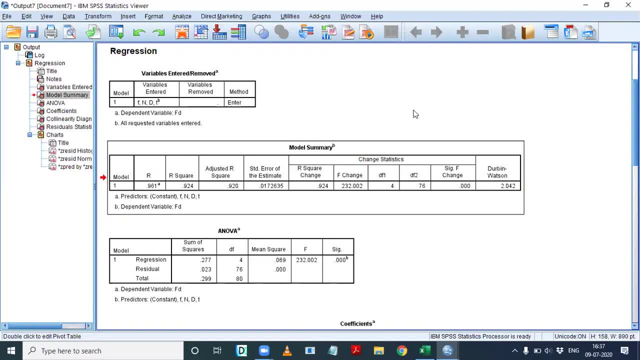 changes. that is here and you have the degree of, you know, 1 and degree of freedom 2. so degree of freedom 1 is nothing but the degree of freedom of T, regression, which is form, because we have four variables, and degree of freedom of T. this is the total degree of freedom. so total degree of freedom is n minus K. 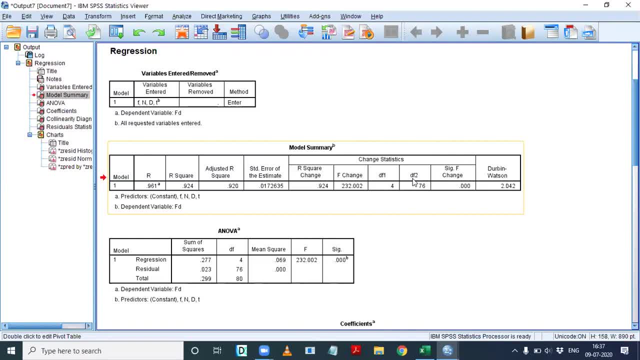 minus one. so you have n minus K. ***N*** is k here, k is the number of variables. 4 minus 1, that is equal to 76. so 81 minus 4 minus 1 is 76. so this is the total degree of freedom and this is the degree of freedom of the regression. 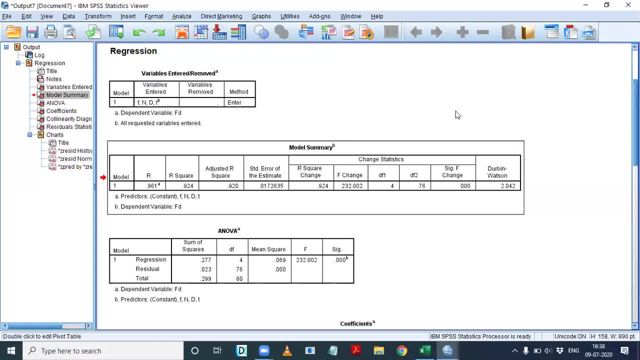 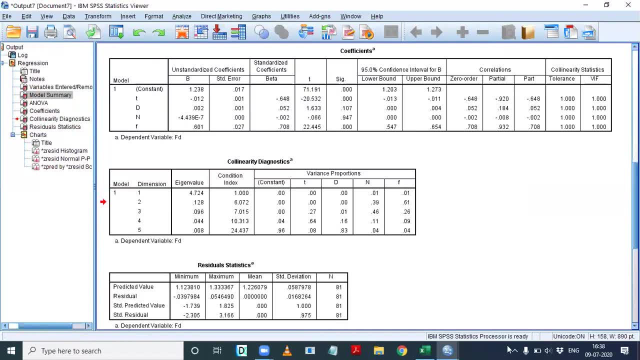 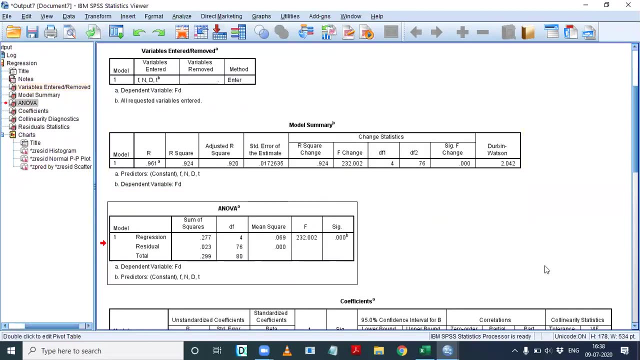 and you have the significant change in the f significance here and you have the durban watson test here. okay, the value of the diagram is interesting and if you look at the- okay, if you look at this, this is nothing but the anova which has been done and in the anova you can see: 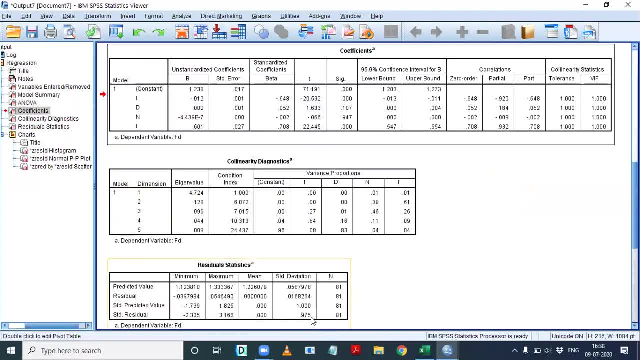 that the model is significant because you have a very low eval. okay, now let us look at the coefficients. so these coefficients make up the regression equation. okay, as you know, these coefficients make up the regression equation, so your regression equation is 1.238 minus 0.12. 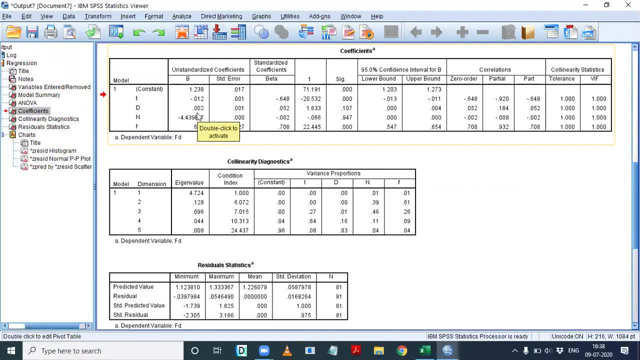 t plus 0.002 d, minus this particular value into n, plus this particular value into f. okay, so this is your regression equation. so this is nothing but the beta naught into the constant. so beta naught is is the constant. so beta naught plus beta 1 t plus beta 2, this is beta 2 d plus beta 3. 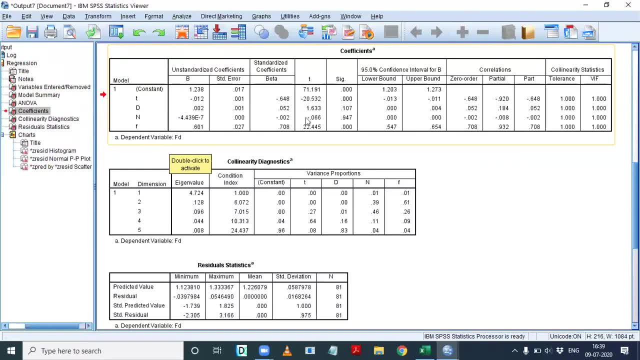 plus beta 4 f. so this is your regression equation and you have the confidence interval bounds here. okay, you see that the bounce for this particular coefficient is between 1.203 to 1.273. okay, so this is the 95 confidence bank. and here, if you look at the collinearity, this is the collinearity diagnostics. so we just want to look at 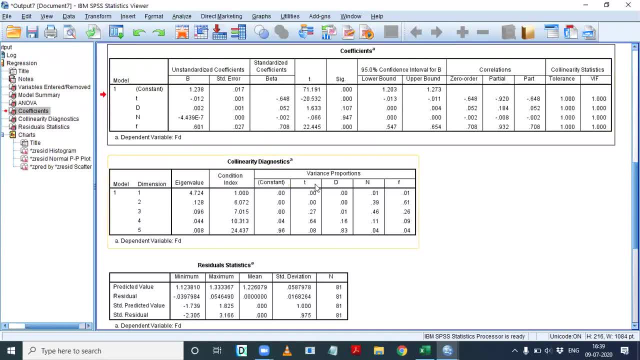 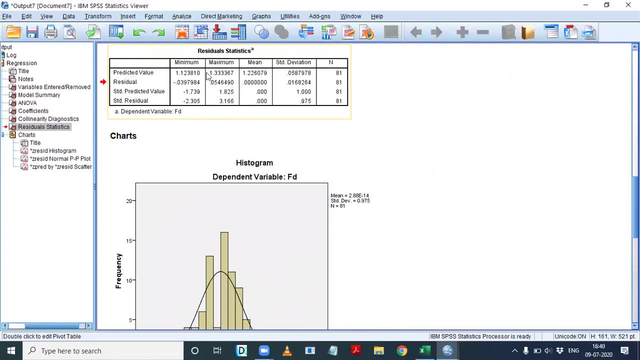 whether the data that you have it has some collinearity or not. if it has some collinearity, we want to avoid that particular quantity from the statistics that you do. now, here you have the residual statistics. in the residual statistics you can see this is the predicted value, is the residual, this is 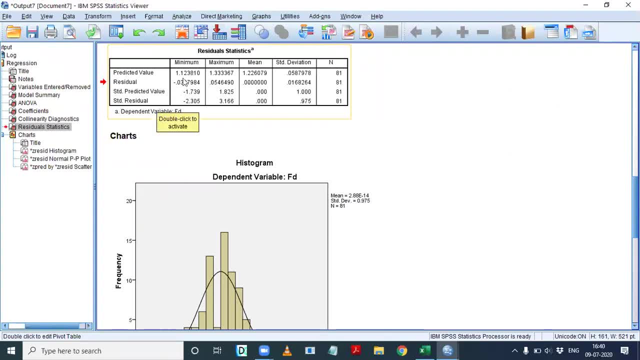 the standard predicted value. this is the standard residual, so this are used. as you have already listened to yesterday's session, where I discussed in detail about the discussed in detail about the, a number of where we discussed about the theory of the regression, in that you have seen this: what are this recently? is the predicted value? what is the minimum? 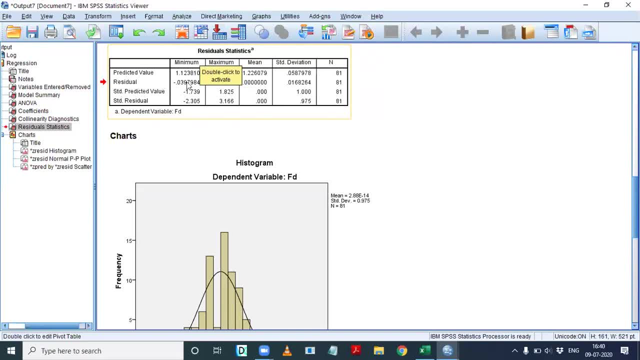 predicted value and maximum predicted value centerssthat. similarly here, what is the minimum residual and the maximum residual and the mean and the standard deviation? all these are so so, as you can see, here n? n is 81 people. we have 81 different samples, so you get 81 different residuals. you get 81 different predicted values. 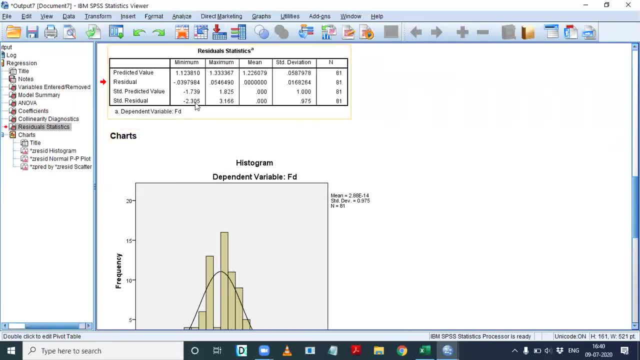 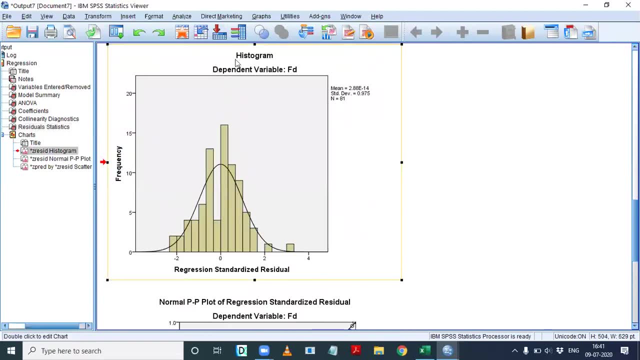 you get 81 different standard residuals. okay, as i told yesterday, you should always look for the standard residuals, okay, and you should not look at the raw residuals, but you should look at the standard residuals. so here you can see the histogram. uh, the histogram is created for the standard residual. so, uh, we have to see that the residual that has been. 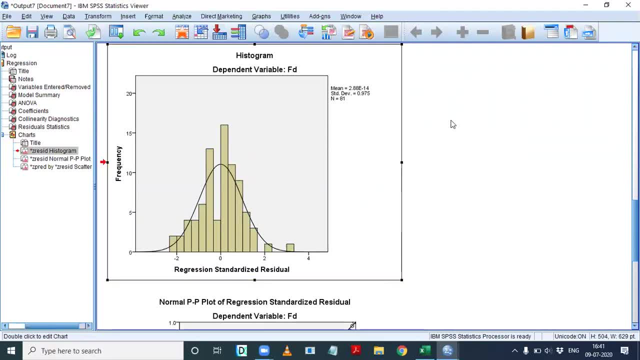 created. that is uh, uh, that is in, in, uh. it is normal or not? okay, if it is normal, uh, if the data, if the uh residual that is generated, that is, that is normal, then we can say that most of the data, uh, or the most of the information from the data, has been extracted. and what? 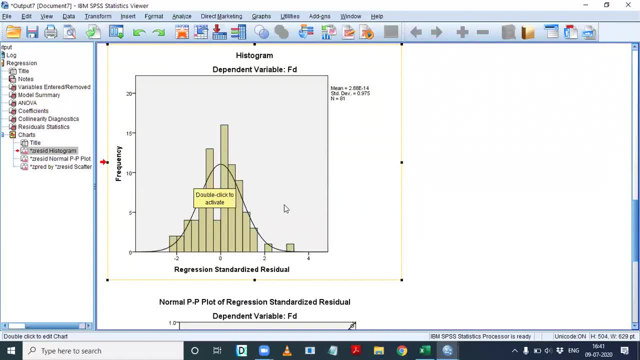 is left behind is the unnew, is the unusable uh residual part. okay, so that is exactly we are trying to see here. next we have the pp plot. i already explained the pp plot so, as you can see, most of the residuals that i have that are kind of lying on this line, but you see some kind of uh furthering. 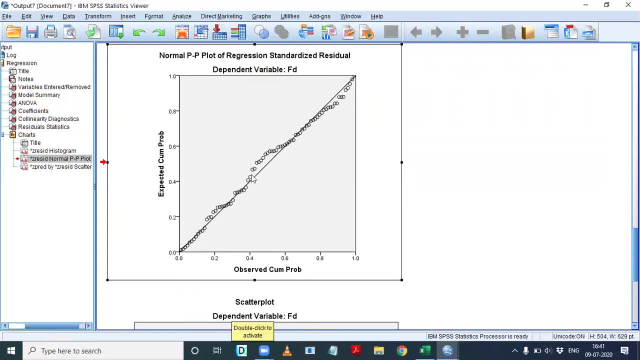 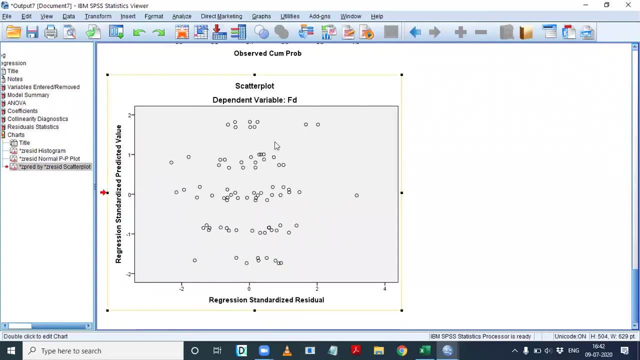 away from this particular line. here and again we can probably do a. we can plot a box plot for this residuals and then we can see if there is any outlier in the uh, in this particular data. then we can go to this plot here. basically, what you see here is that this is the standardized 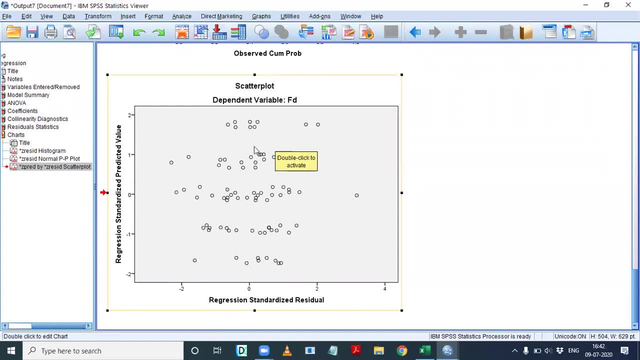 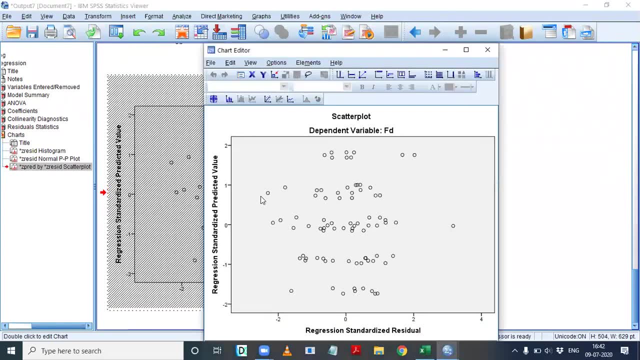 swimming start, which is the standardized uh regression. okay, so here what should happen is that no kind of uh pattern should form. okay, so if you double click here and if you go and try to uh form a regression line for this particular data, then you should not be. 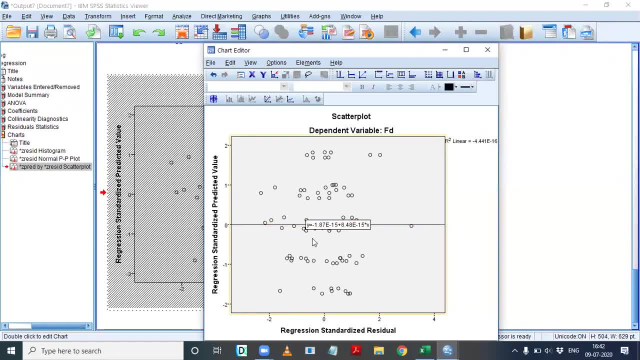 able to, you should not be able to get any regression line. as you can see, there is no regression line here. the relation line is flat. so, you see, do not see any trend here. you do not see any upward trend or downward trend or anything else. okay, so what i mean to say is that whenever 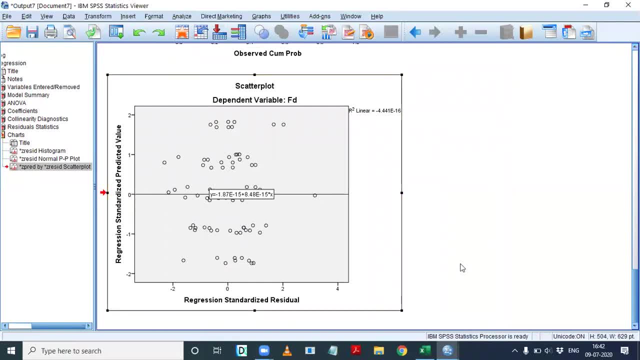 you analyze the residuals, there should not be any trend, okay, there should not be any uphill trend or downhill trend, and all that. so this is a very, very important kind of plot that you should always generate, along with the, along with the regression that you are doing. okay, now 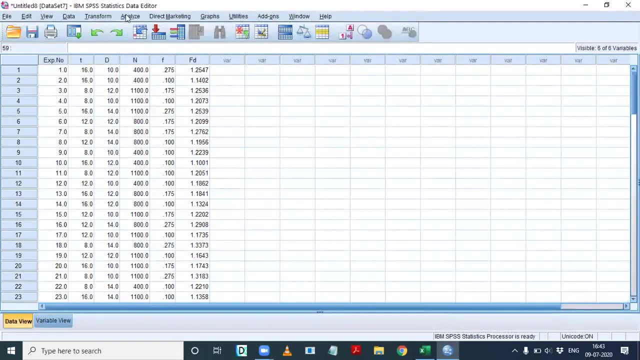 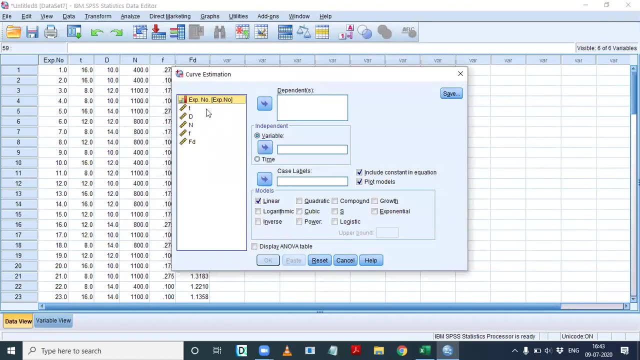 let us just close all of this and let us go here again and let us again go to regression, and this time we will go for curve estimation. in the curve estimation, what we will try to do is that if this curve estimation is nothing but same as the regression, but here, 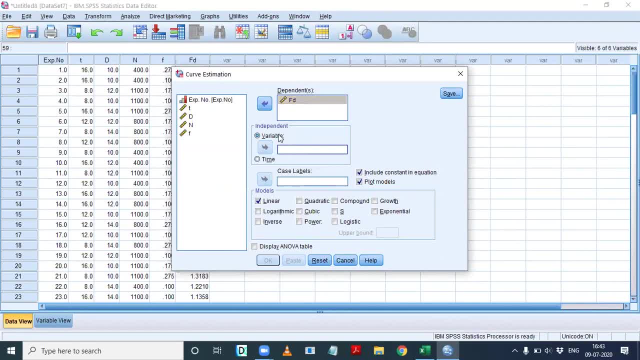 what we'll do is that we can go with one variable at a time. okay, you can go with one variable at a time. imagine that this is a univariate problem. in that case you can go for. uh, in that case you can go for curve estimation. suppose, say you have. 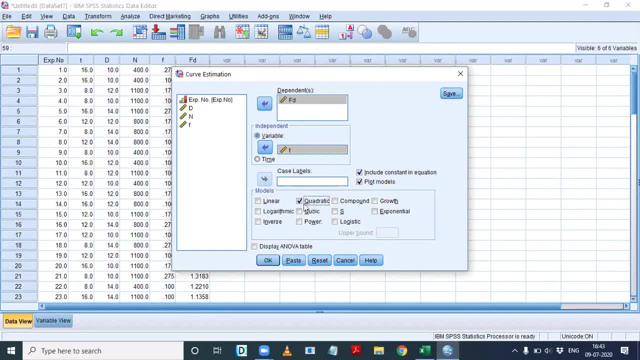 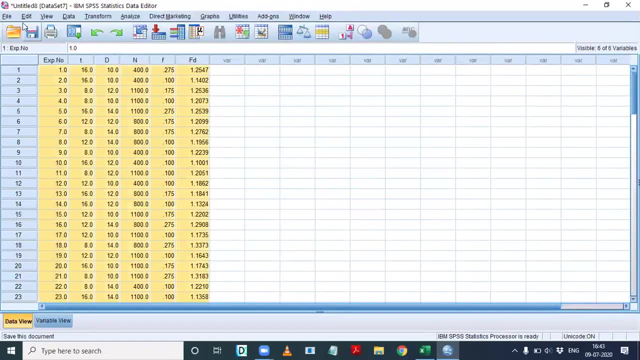 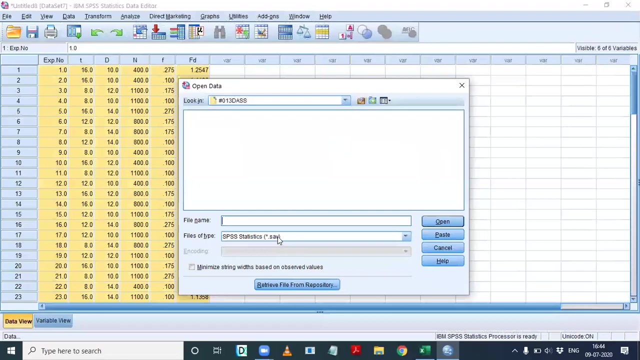 already seen the linear. instead of that, if you suppose say want to go for this one, this is suppose say: okay, let me not work on this particular data set and let me work on some other data set. okay, open data set. new query search open. because i do not want to confuse you by taking a. 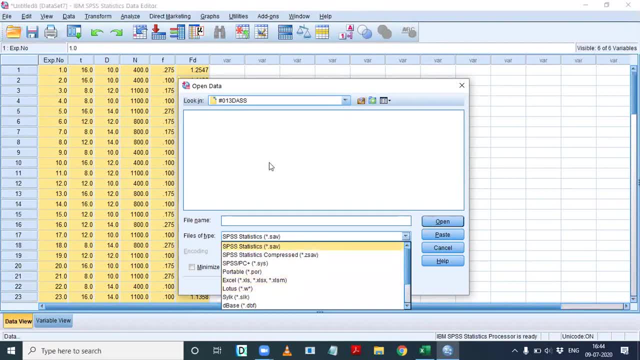 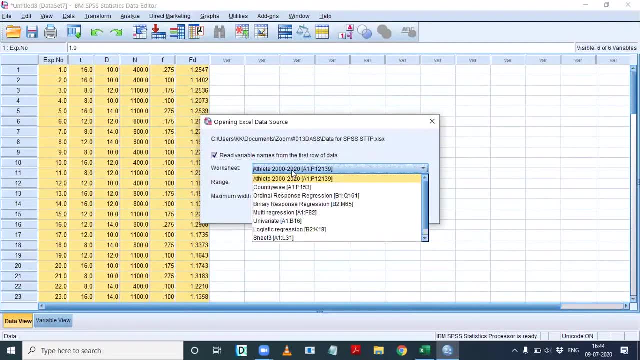 univariate out of a multivariate which is actually in multivariate. i do not want to take any univariate example out of it, so i want to have a univariate sample. i think i have one here. better still, i have this: go with this one. i have a univariate data. 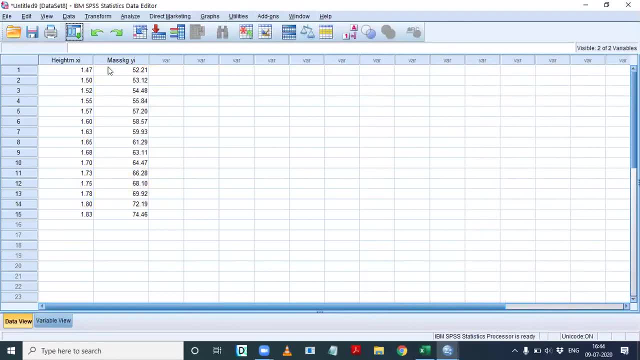 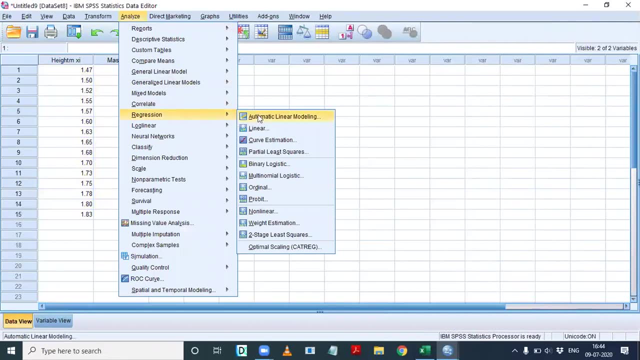 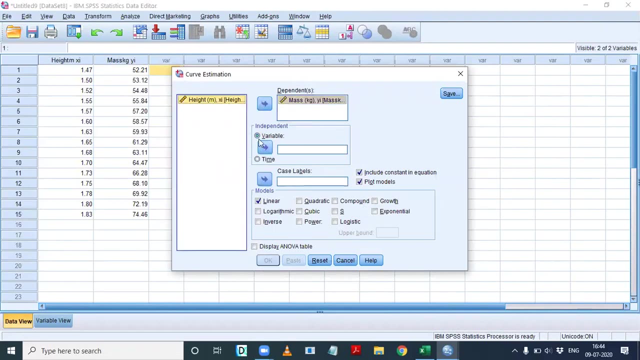 here. okay, this is the univariate data for height versus the mass of the female convenience, height versus the mass of the female candidates. so here, if i want to analyze, if i can go to this curve estimation, i can go and select the dependent as the mass and i can go and select the height as the independent. 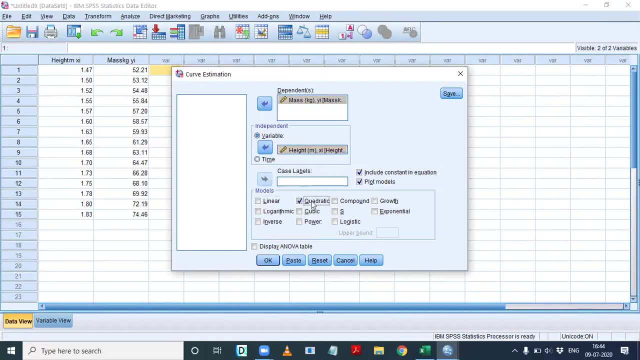 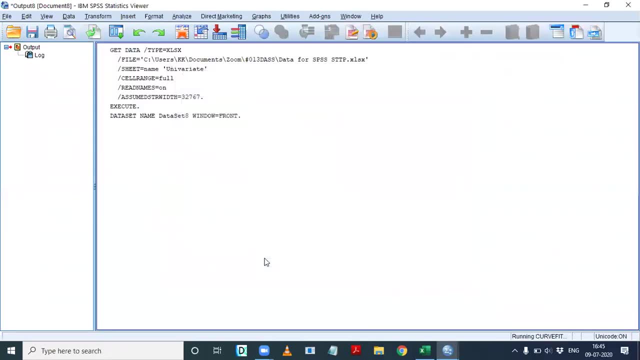 and now i want to go, for suppose, say, quantity quadratic means a second order, okay, and i want to get the uh enoba also. so i'm going to go and click on this, i'm going to one click, okay, so you can see if you want to take um, anoma is equal to a f or n, and so if you want, 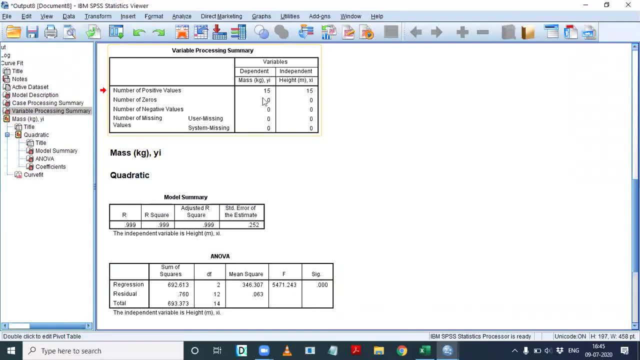 see that there are 15 different cases, and all of these 15 different cases, all of them have positive values. okay, and here, what do you see? you have a r square of 0.99, almost one, and this adjusted r square is also one. okay, meaning very high, kind of. 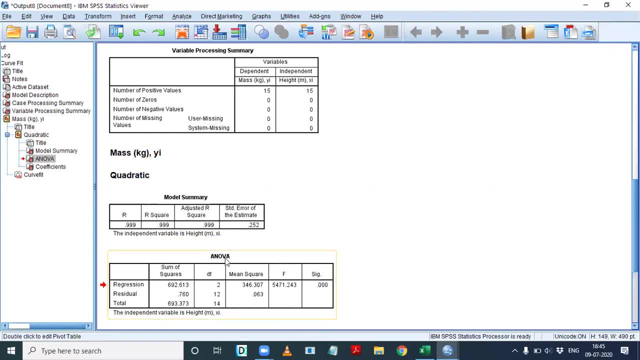 very low variance, negligible variance in the data. okay by s as seen by this model. okay, so we have the anova here in. the anova also says that the model that we have done or the iteration that we have done is significant. now let us look at the 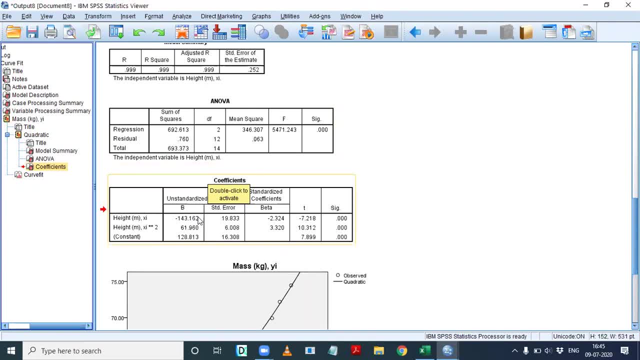 coefficients: okay, these are the coefficients that we have. as you can see, these are the coefficients that we have and in the coefficients you can see, since it is a second order model, so our equation is: uh, beta one. okay, our equation is nothing but mx plus c plus. 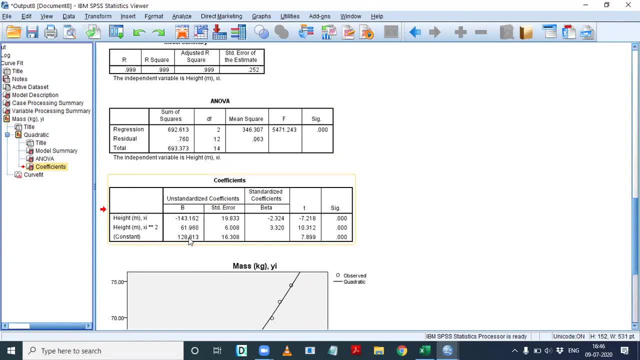 into. suppose say n x squared, okay, we have. m suppose say we have c plus mx plus n x squared. or we can say that we have we gone out plus beta one x plus beta two x squared. that is what we have here. this is beta naught plus beta 1. 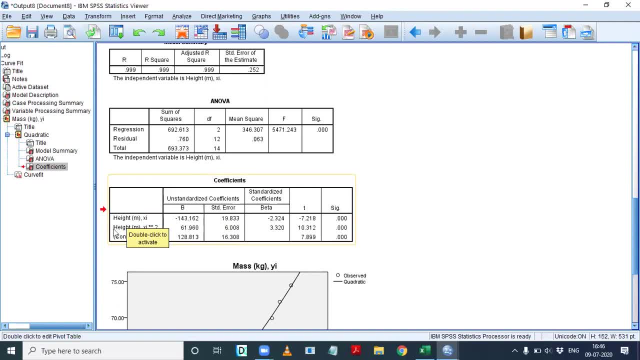 into height plus beta 2 into height squared. okay, so we have beta naught into into, uh, beta naught plus beta one x. okay, my question is your c is what you call plus beta to x, squared. okay, that is exactly what we have here, okay, so? 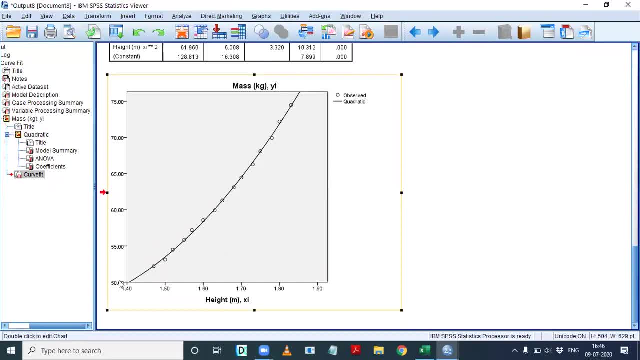 and we can go and look at the curve fit also, you can see that, uh, it's, it's, it's kind of a very, very nice fit. yesterday, when i used the same data for having a uh linear line or a uh or a first order- in fact this is also linear. so what uh in yesterday's example, when what we? 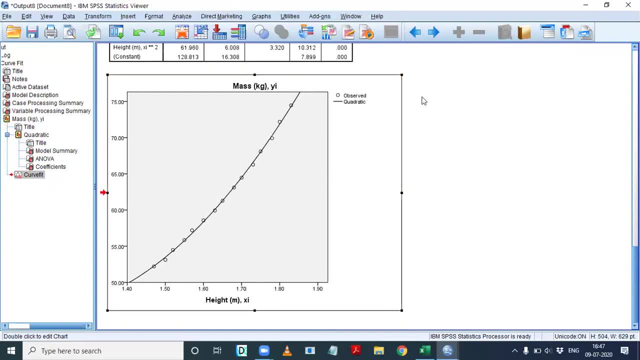 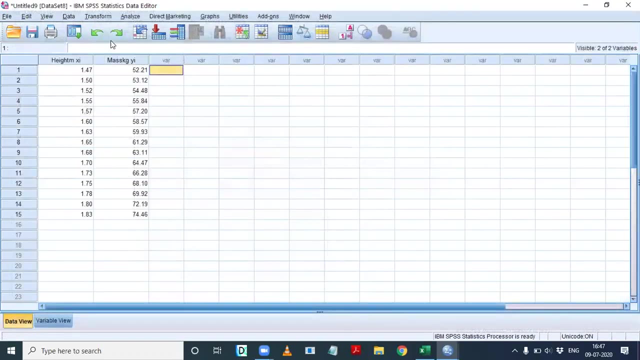 had was that we had one uh straight line in that case. uh, we saw that uh d line was not passing to all the points. but here you can see the line discussing kind of passing through all the points. okay, so we'll go and use the same data set again for some other analysis. i want to look at the 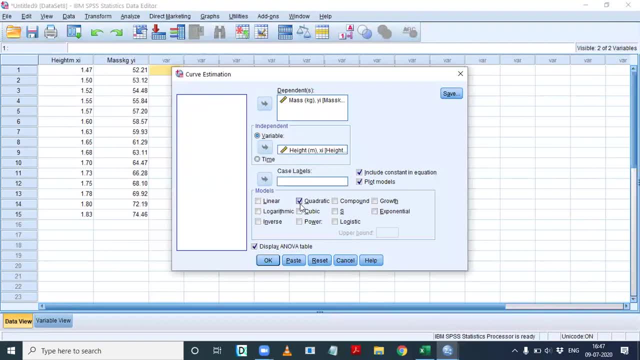 other regression also. so here, instead of suppose, say, the quadratic, you can go for suppose, say, though exponential may give a weird kind of result. so but let us go, for the sake of understanding, let us go and see what happens when we try to fit a exponential curve on this particular data set. 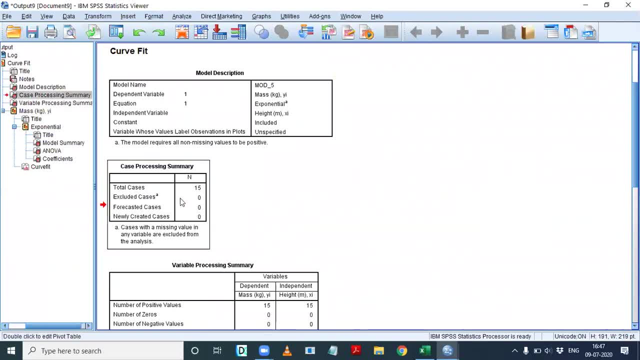 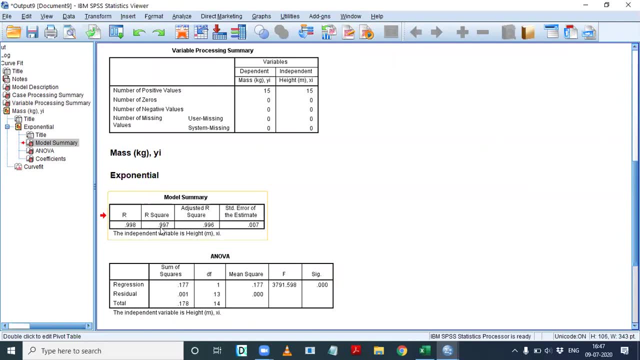 or a exponential regression we want to do on this particular data set. so what will happen? okay, all these are same. so you can see that now my r square kind of has decreased because, as you know, if i go up in the exponential series, what will happen is that my 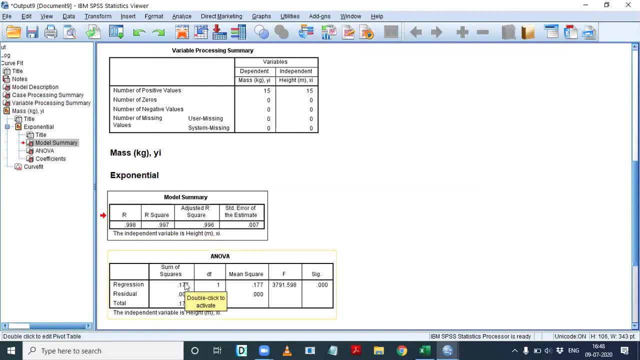 curve will become sharper and sharper. my increase in the curve will become sharper and sharper, though still, the anova is showing that the model is significant, which is also you can see here that, uh, the r square, the change in r square is not that huge, means the adjusted r square is not dropped. 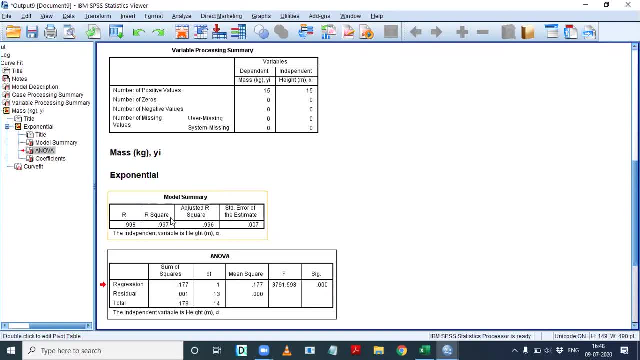 okay, as compared to the r square. okay, here i want to give you another, uh practical tip. the practical tip is that whenever you conduct a regression in any kind of regression- okay, it may be logistic regression, it may be, uh, univariate, it may be logistic regression, it may be, uh, univariate- you 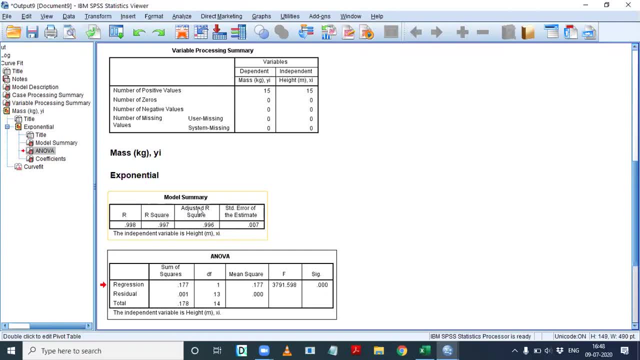 may be motivated whenever you see that this is the r square and whenever you see that this is supposedly adjusted r square if you see a more than 20 drop. okay means what i mean to say is that if you say that this is 99.7 percent and this is 99.6 percent, it's perfectly okay. okay if you're. 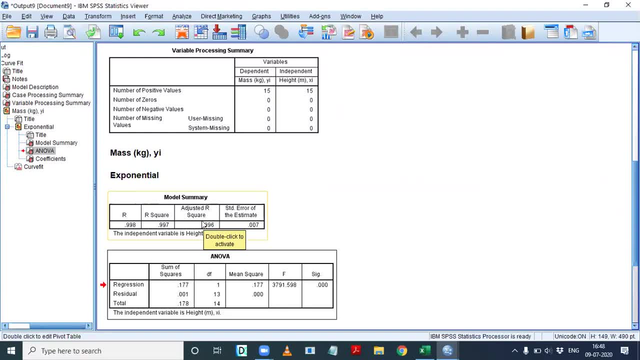 supposed to say this is 99.7 percent, and if you see a drop in the adjusted r square of more than 20 percent, then you should be a little careful of that model, because that model has now some unwanted factors in it- okay, or some unwanted uh variables in it okay. so always trying to see that the 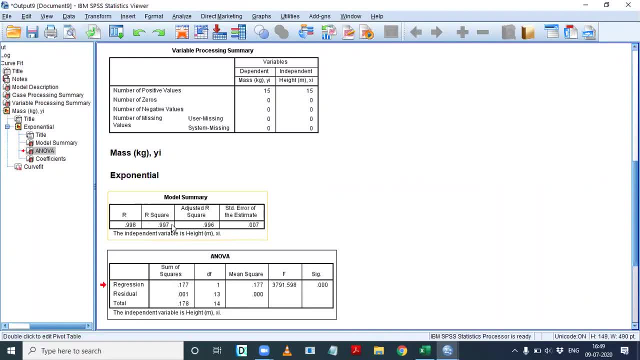 difference between these two is not more than 20. if suppose that this is 99.7 and then somewhere around 79.7 is okay. if it falls below 79.7 percent for the adjusted r square, then probably there is some problem with the analysis that we have done. just go and see the anova and then i. 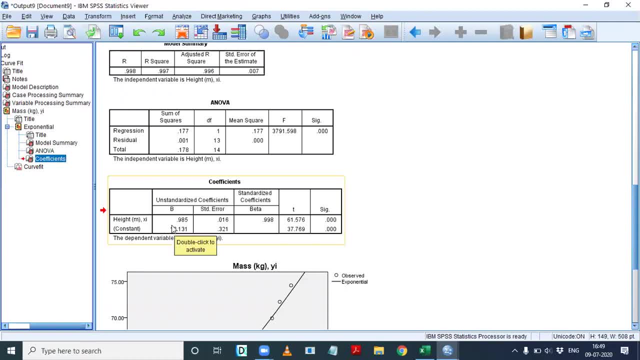 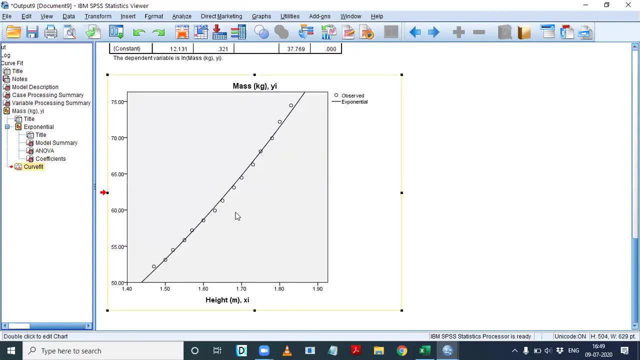 can go and see the coefficients. as you can see the coefficients, okay, the coefficients are here. uh, you have the constant and you have the high and if you want to, okay. so if you can see that here after, if the curve will kind of, uh, try to move away. 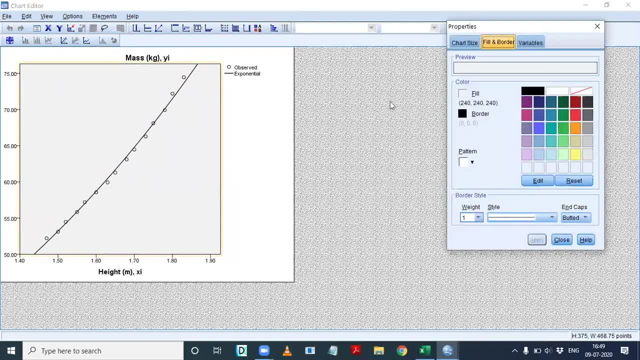 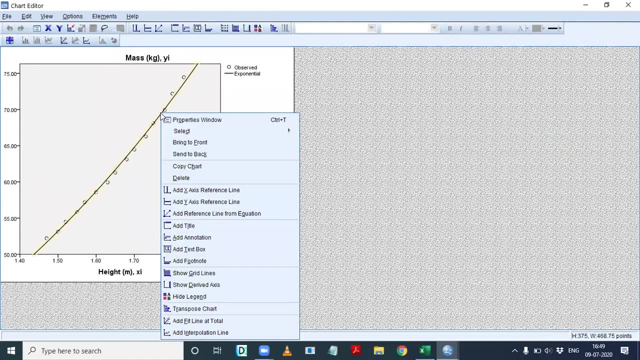 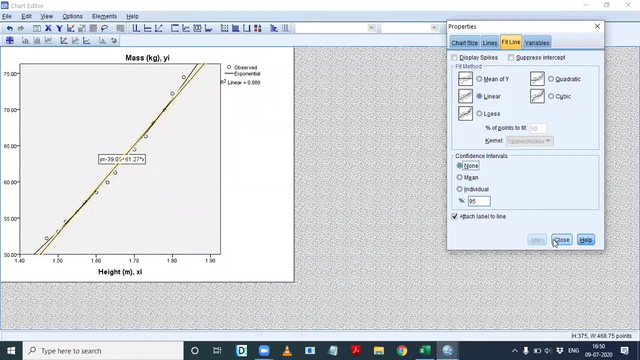 and okay, i just wanted to show you this. okay, that how it differs from it, this line. let me put it in red and let me increase the width of this line, and let me increase the width of this line and let me increase the width of this line. 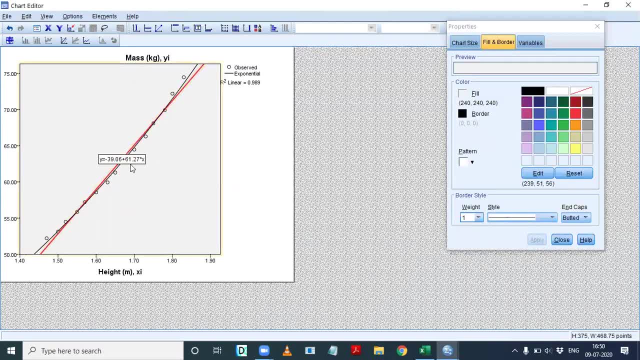 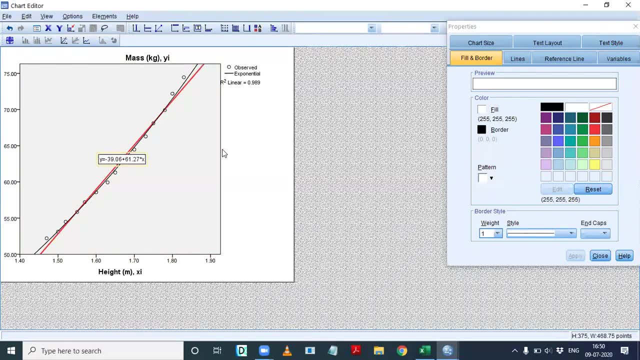 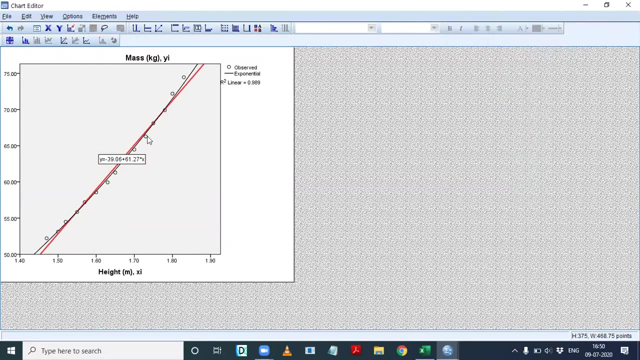 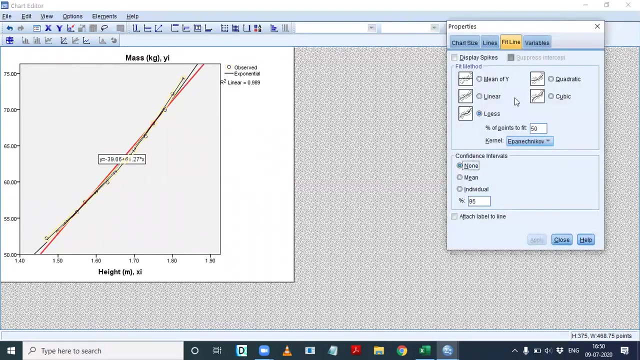 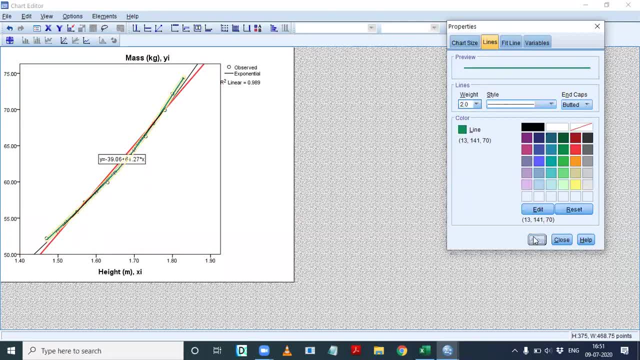 and, and i will decrease the size, the first part then. so you go and look at all the parameters and these two different types of length. this line changes the amount of方面, these two beta, uh, this line, this time suppose any quadratic line. let me put this line in some other color, so as you. 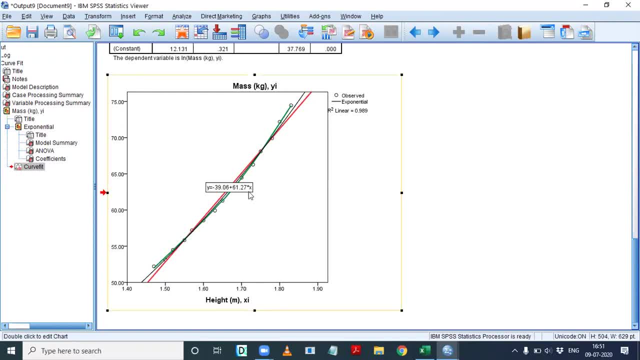 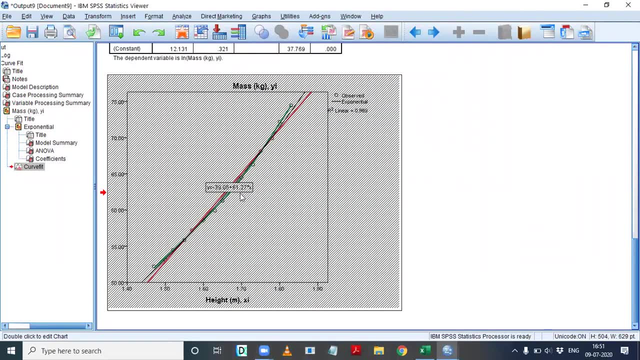 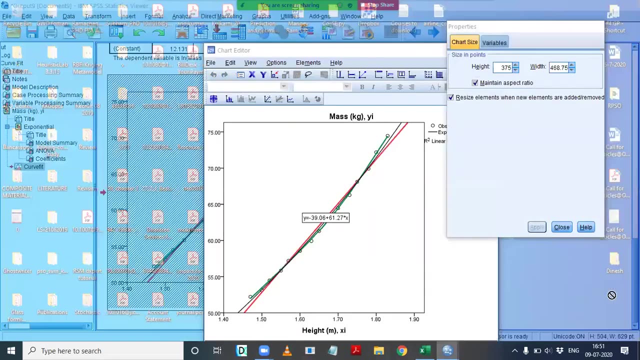 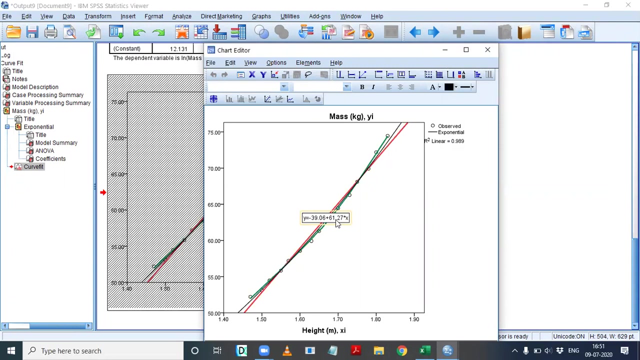 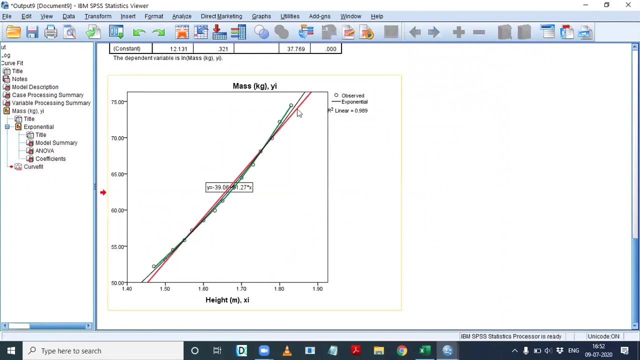 can see here, just deleted this one. okay, it's. what is it? what is here? let me close this this one. okay, okay, okay, okay, okay, okay. so, as you can see here, this is the three different kinds of curves that you see here. so this green one is the second order line, or the 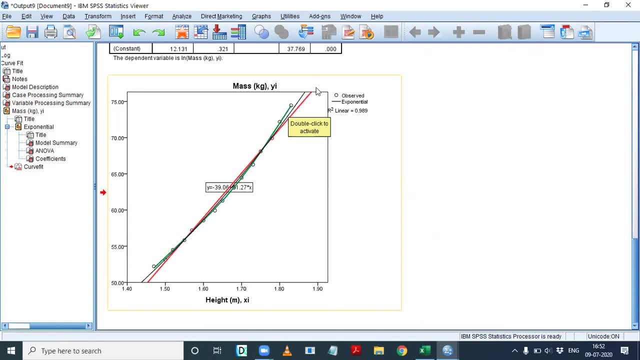 quadratic line. this red one is the straight line, or the first order line, or the linear. this is D, this one, the middle one, is the kind of the exponential curve. so like this also, you can compare and see which line gives you the kind of the best result. but as you, as you can probably tell with the help of the R square, 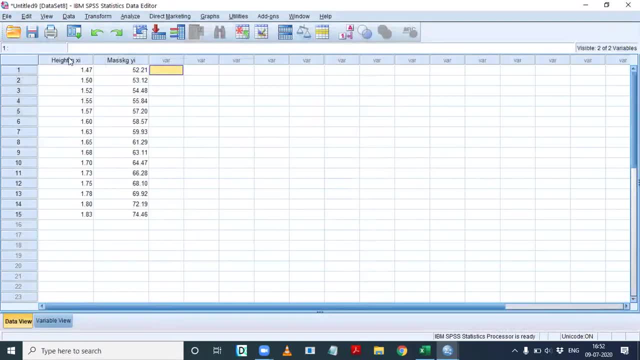 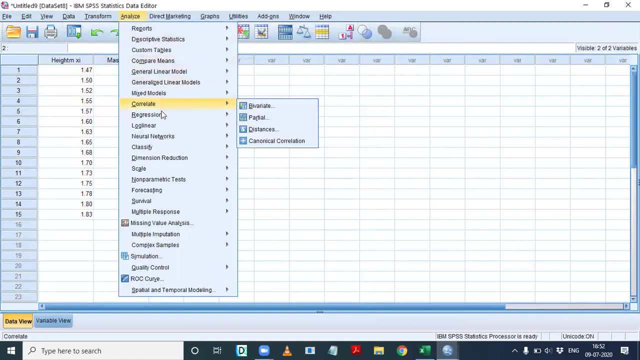 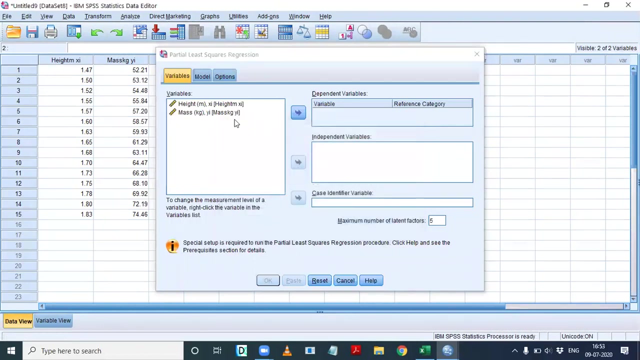 itself that the perhaps the second order line or the second order equation was kind of the best one for this particular data set. and we have some other kinds of regressions also, for example, I'm not sure with this data, the partial least squares. so if suppose, say, the mass is your dependent one and 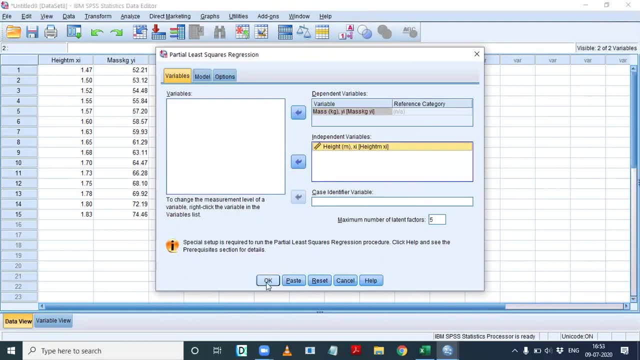 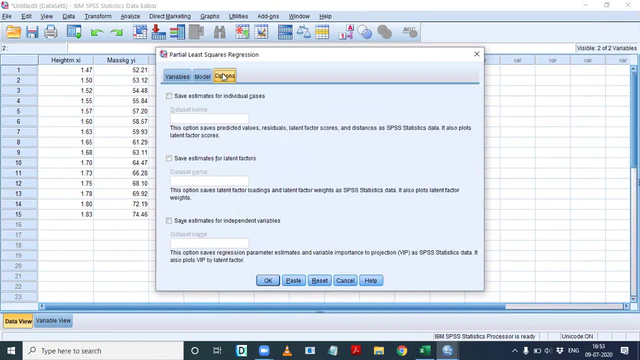 height is your independent one, and then click, you go to the model and you want to suppose, say you want to look at the measurement and you want to look at the measurement and you want to look at the main effects you have. you can save on main effects you have. you can save on. 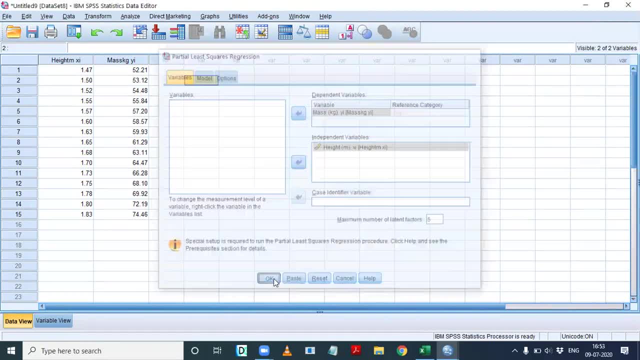 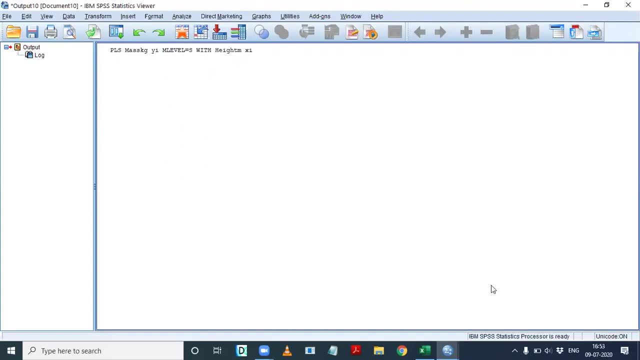 main effects you have. you can save on this and you're going to save on this, this, and you're going to save on this, this and you're going to save on this right now, right now, right now, I may have some module that is missing from my data, from my guess spaces, because 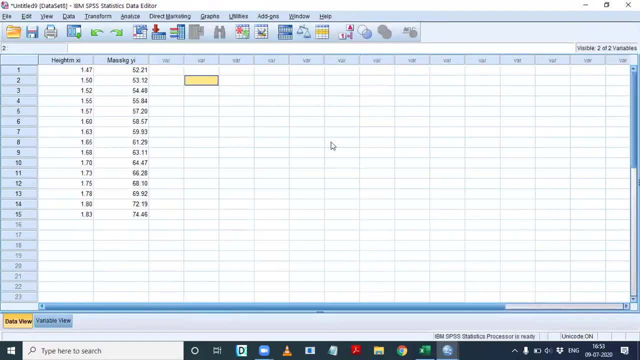 I may have some module that is missing from my data, from my guess spaces, because I may have some module that is missing from my data, from my guess spaces, because of which it is showing, of which it is showing, of which it is showing some kind of error. but anyhow, we'll see some. 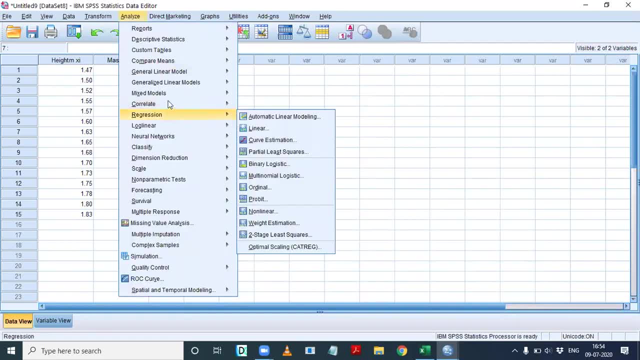 some kind of error, but anyhow, we'll see some some kind of error, but anyhow, we'll see some examples of the don't worry, we'll see examples of the don't worry, we'll see examples of the don't worry, we'll see some examples of the g-square tomorrow. 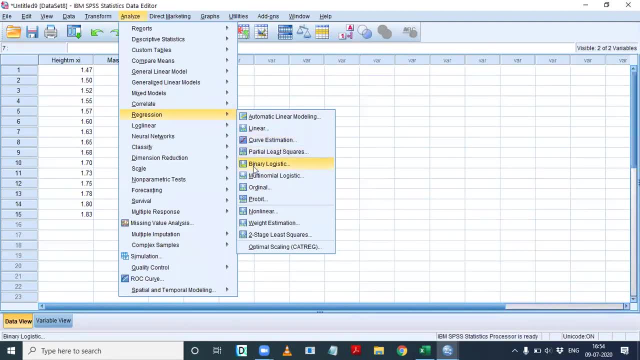 some examples of the g-square tomorrow. some examples of the g-square tomorrow: because I have some special data that I, because I have some special data that I, because I have some special data that I have loaded for the e-square and then we have loaded for the e-square and then we 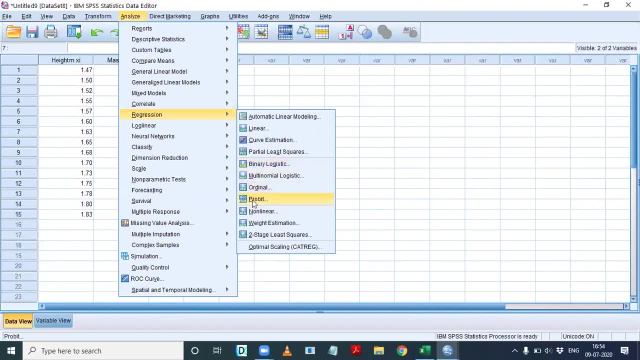 have loaded for the e-square, and then we look at something called the ordinal, look at something called the ordinal, look at something called the ordinal data set and we look at ordinal data set and we look at ordinal data set and we look at ordinal regression and we look at binary. 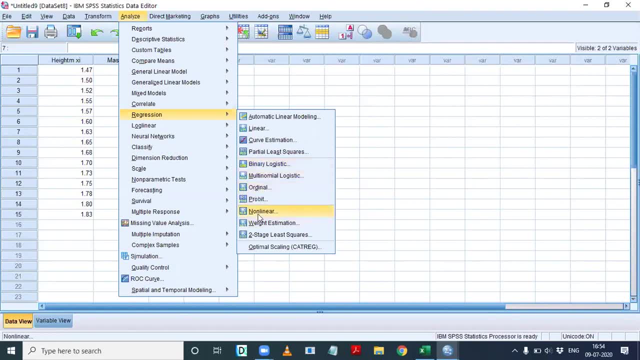 regression and we look at binary regression and we look at binary logistic regression model and we look at logistic regression model and we look at logistic regression model and we look at the nonlinear regression also. so I think the nonlinear regression also, so I think the nonlinear regression also. so I think we can stop this session here for today. 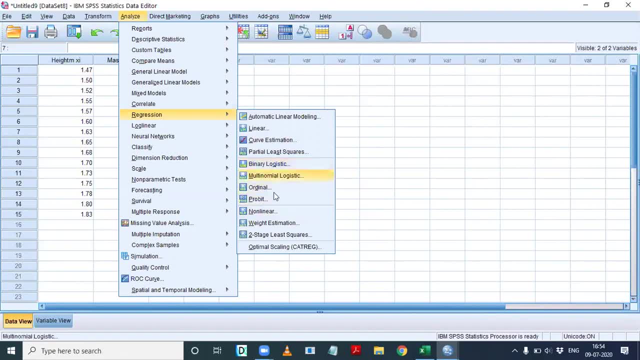 we can stop this session here for today. we can stop this session here for today and tomorrow. we will see with some of, and tomorrow we will see with some of, and tomorrow we will see with some of the important, other other kind of the important, other other kind of. 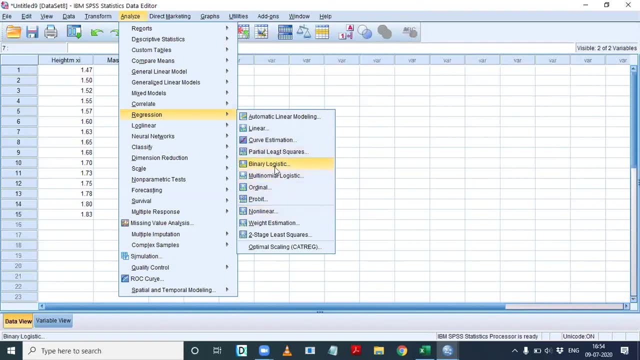 the important other other kind of regressions that are there and for all regressions that are there and for all regressions that are there and for all these regressions, you need some kind of these regressions. you need some kind of these regressions. you need some kind of special data, for example in ordinal you. 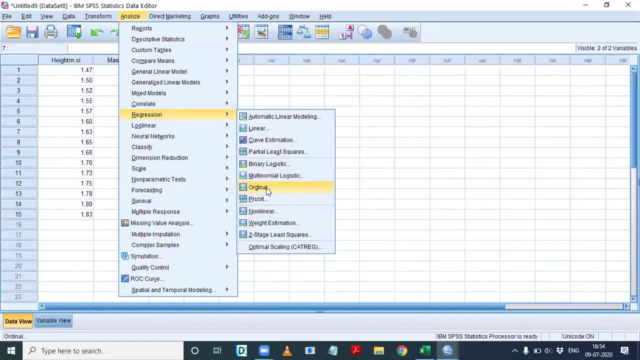 special data, for example, in ordinal you. special data, for example, in ordinal you, need data where some of the data is in need. data where some of the data is in need. data where some of the data is in ordinal scale means it is in order by. ordinal scale means it is in order by. 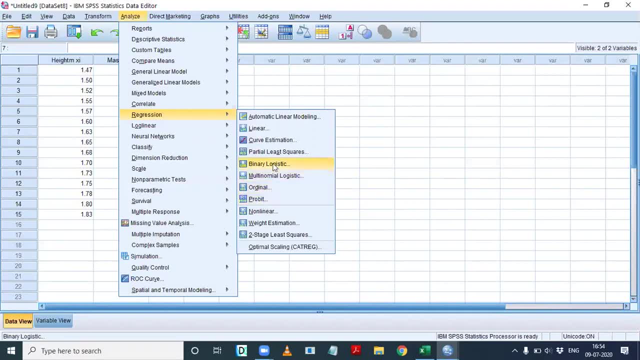 ordinal scale means it is in order by scale. in binary logistic scale, it also scale in binary logistic scale. it also scale in binary logistic scale. it also works well when you have some binary. works well when you have some binary. works well when you have some binary data and you have multinomial logistic. 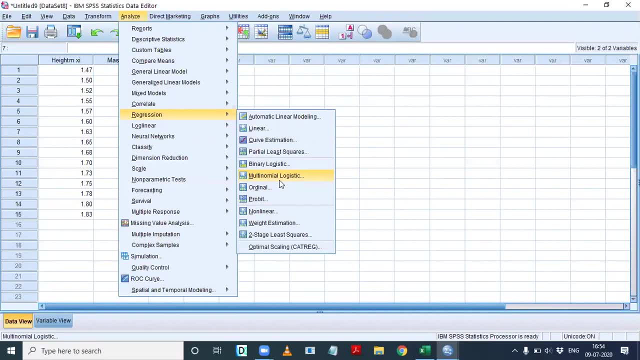 data and you have multinomial logistic data and you have multinomial logistic, so where you have multiple data, which, so where you have multiple data, which, so where you have multiple data which are nominal means they are in terms of are nominal means, they are in terms of.